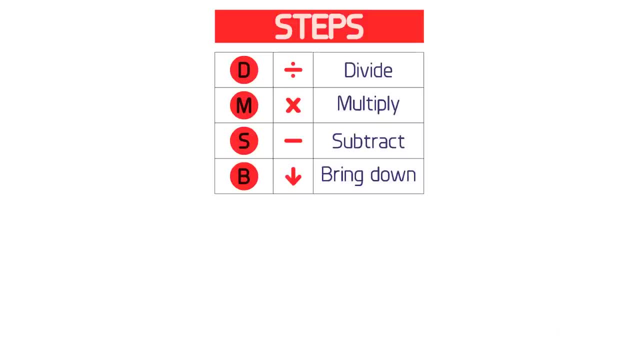 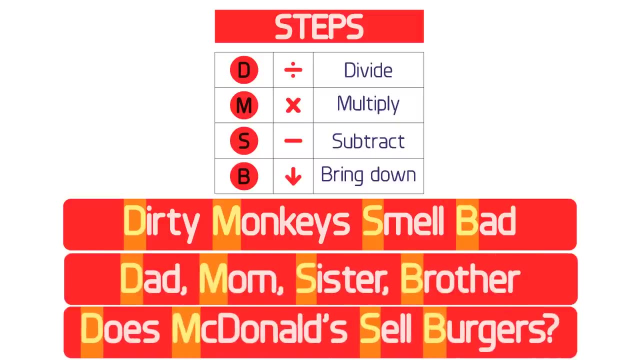 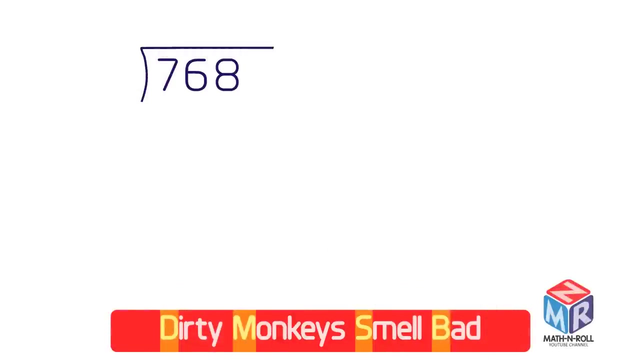 is an easy way to remember the steps of long division. Use any of these Dirty monkeys smell bad. dad, mom, sister, brother, or does McDonald's sell burgers? Let's divide 768 by 3.. To begin ask how many times 3 goes into 7.. 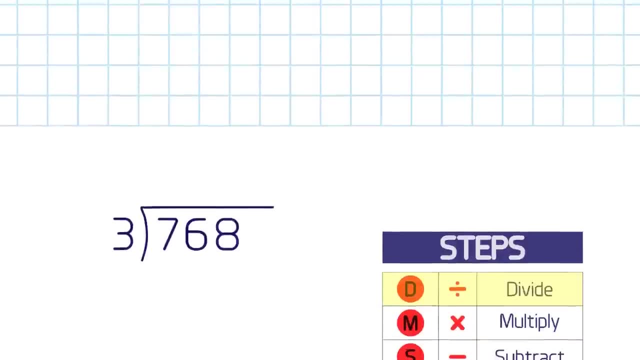 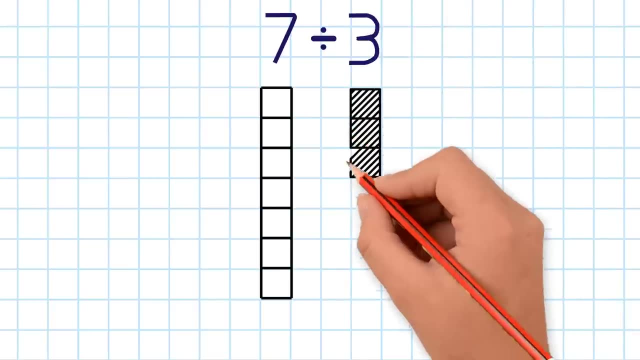 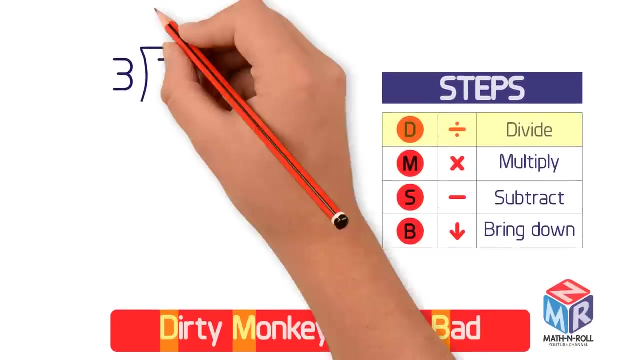 That is, what's 7 divided by 3?? The answer is 2, with a little leftover. So write 2 directly above the 7.. Now multiply 3 by 2 to get 6.. Place the product directly below the 7 and draw a line beneath it. Subtract 6 from 7 to get 1.. 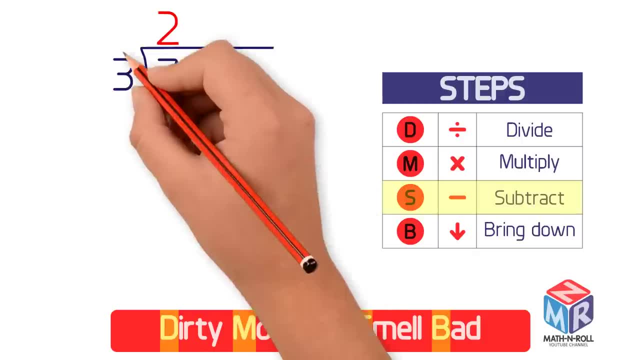 After you subtract, the result should be less than the divisor. In this problem, the divisor is 3.. 3 is less than 1, so it's okay. Then bring down the next number, 6, to make the new number 16.. 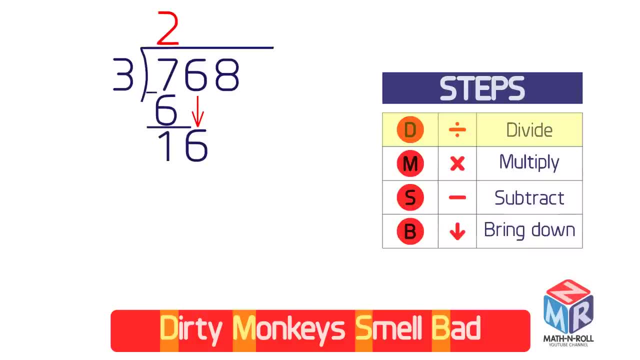 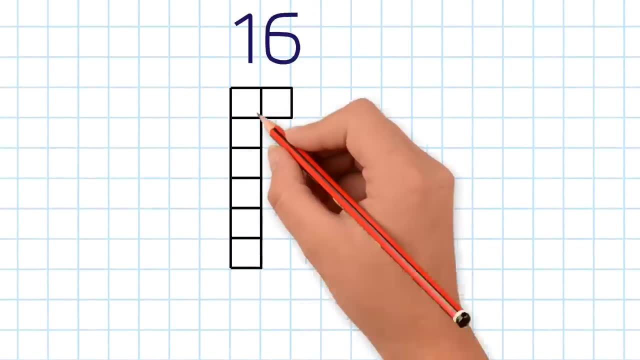 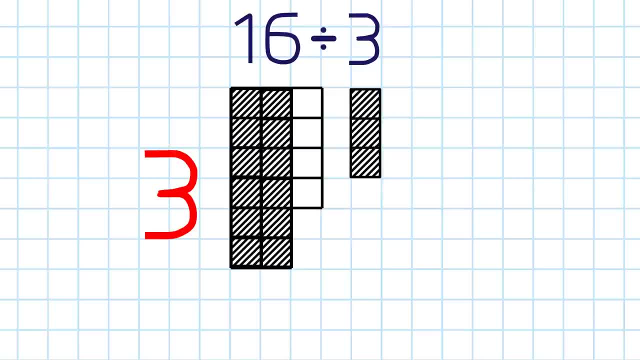 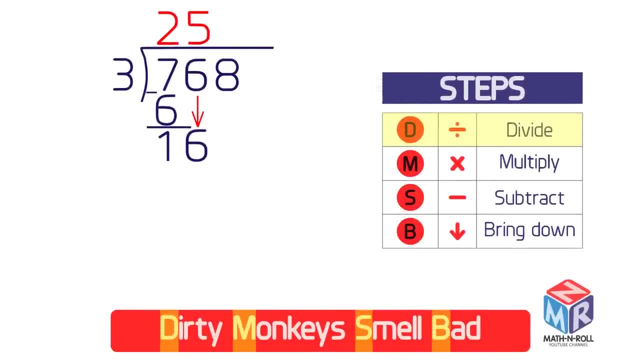 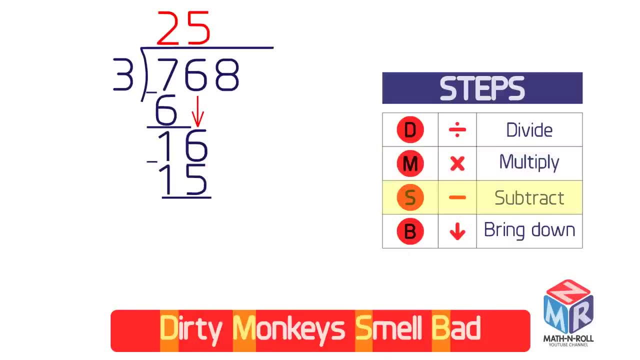 Subtract 15 from 16 to get 1.. After you subtract, the result should be less than the divisor. 1 is less than 3, so it's okay. Then bring down the next number, 8.. To make the new number 18.. 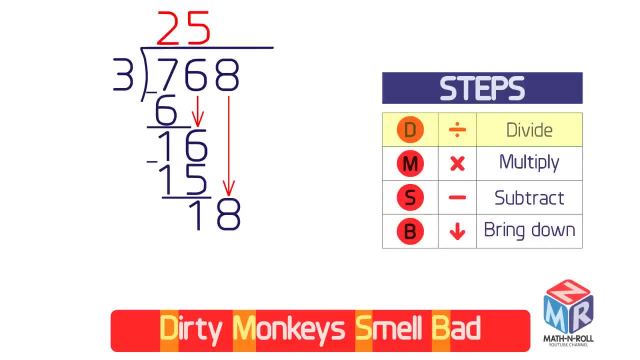 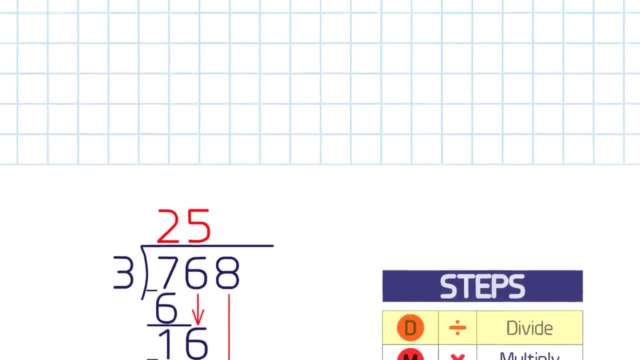 Another cycle is complete, So begin the next cycle by asking how many times 3 goes into 18.. That is, what's 18 divided by 3?? The answer is 2.. The answer is 2.. The answer is 2.. 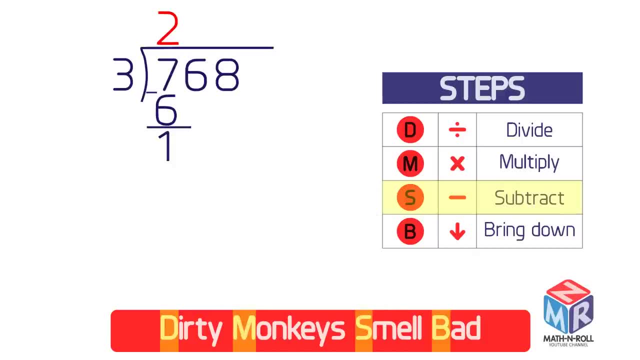 After you subtract, the result should be less than the divisor. In this problem, the divisor is 3.. 3 is greater than 1.. So it's okay. Then bring down the next number, 6, to make the new number 16.. Now ask how many times 3 goes into 16.. 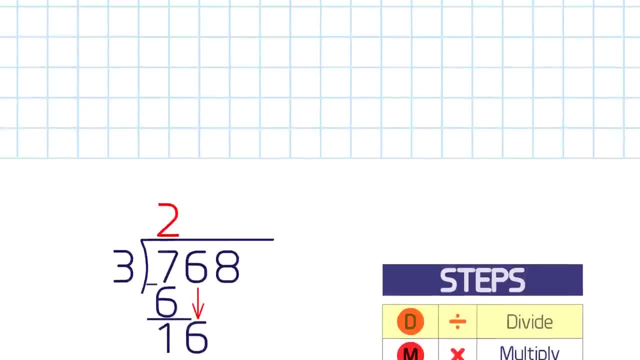 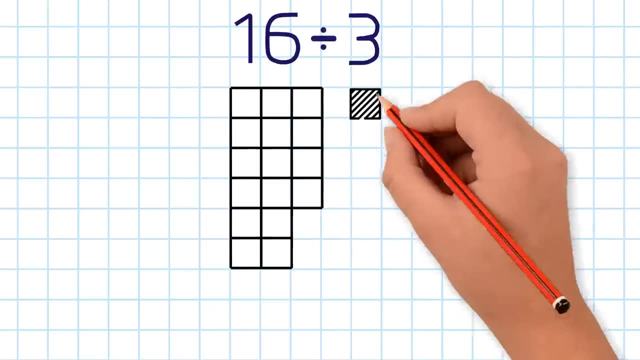 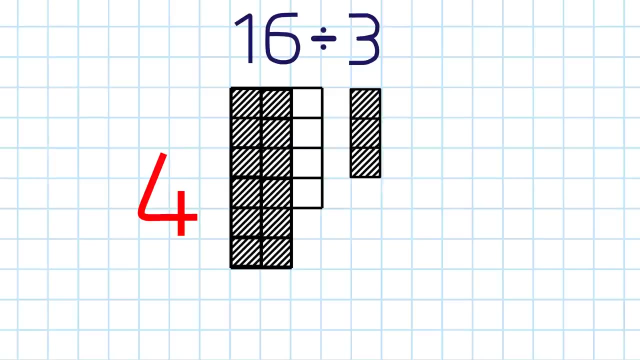 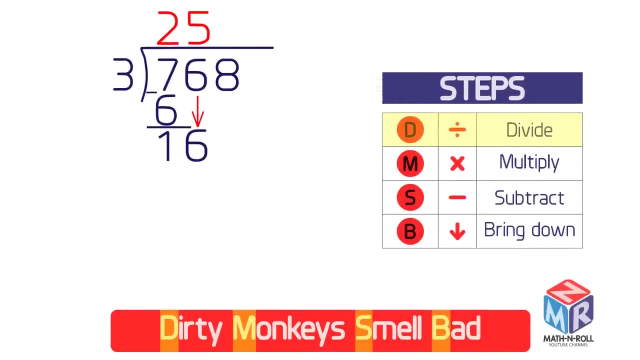 That is, what's 16 divided by 3?? The answer is 2.. The answer is 5, with the remainder. So write 5 above the 6. Then multiply 3 by 5 to get 15.. Write the product under 16.. Subtract 15 from 16 to get 1.. 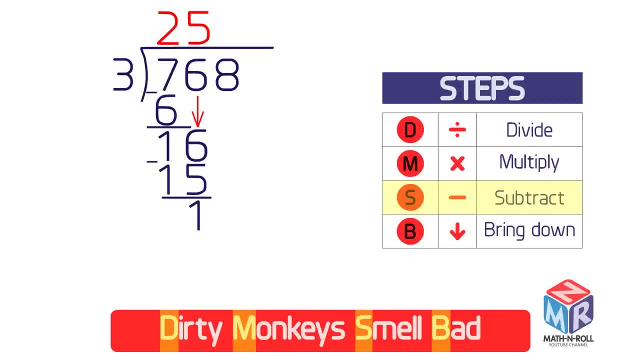 After you subtract, the result should be less than the divisor. 1 is less than 3.. So it's okay. Then bring down the next number, 8, to make the new number 18.. Another cycle is complete, so begin the next cycle by asking how many times 3 goes into. 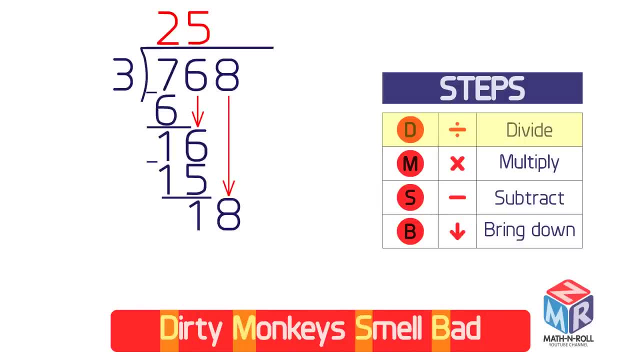 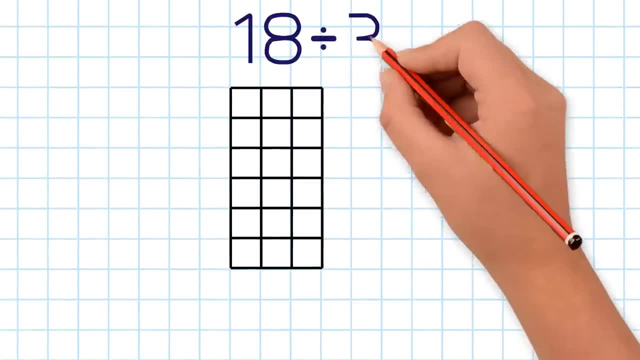 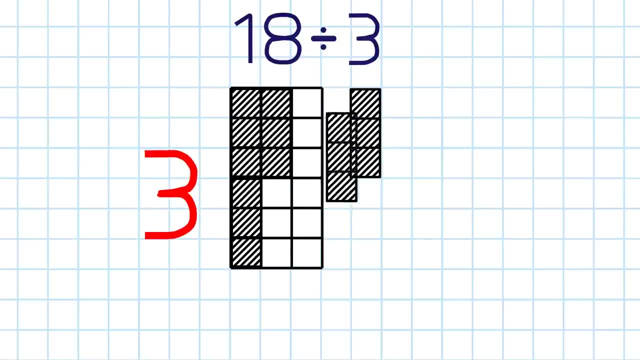 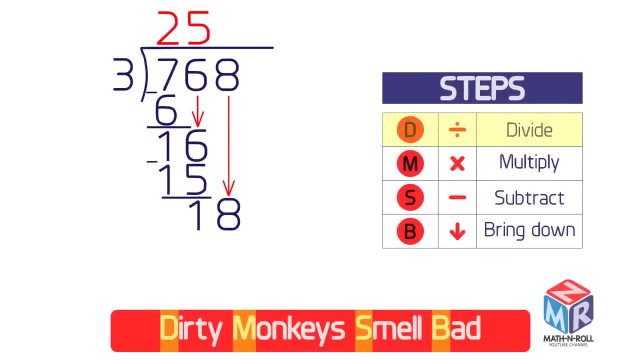 18,. that is, what's 18 divided by 3?? The answer this time is 6.. Write down 6 above the 8,, multiply 3 by 6, and place this below the 18.. Now subtract 18 from 18 to get 0.. 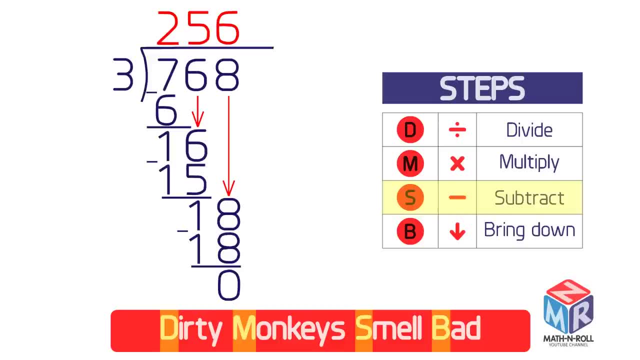 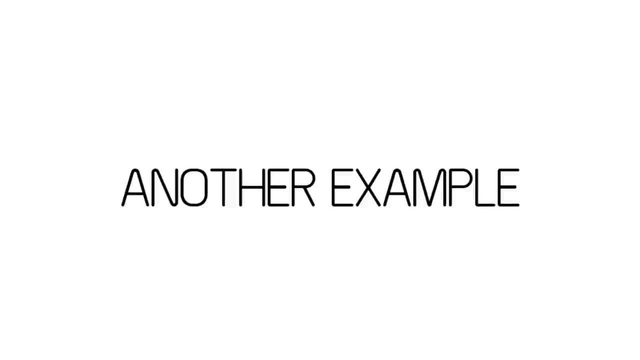 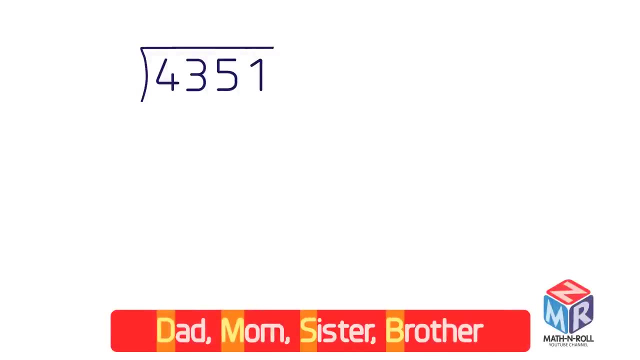 Because you have no more numbers to bring down. you are finished and the answer is 256.. Thank you. Let's try another example. Divide 4,351 by 6.. To begin ask how many times 6 goes into 4?. 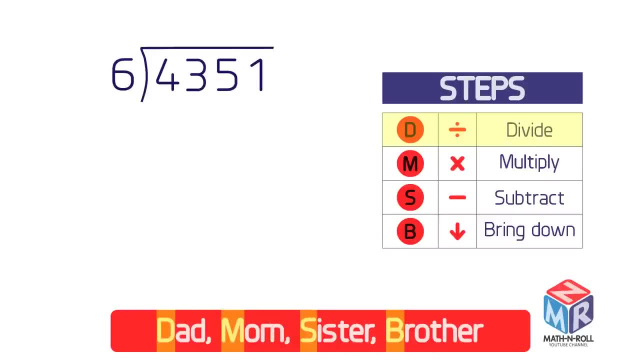 None. That's because the first digit taken by itself is less than the divisor. 4 is less than 6.. Write 0, or just leave a space above the 4.. Let's group the 4 and the 3 together. 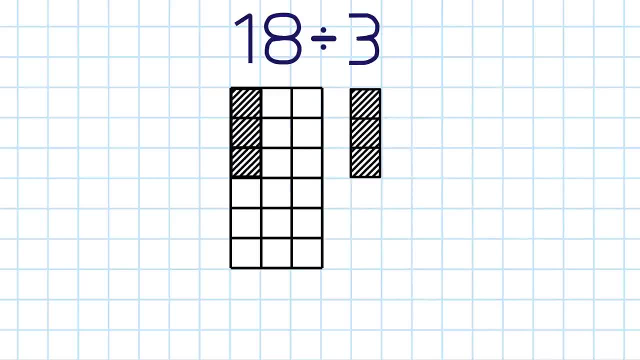 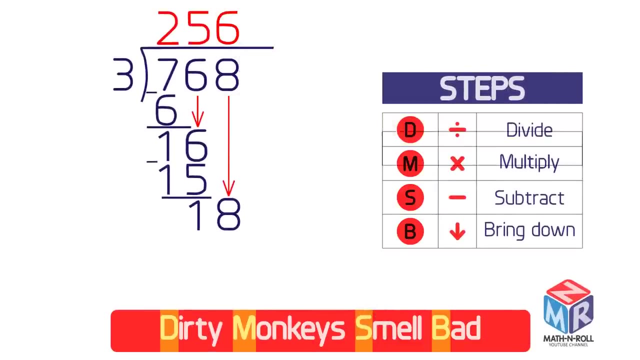 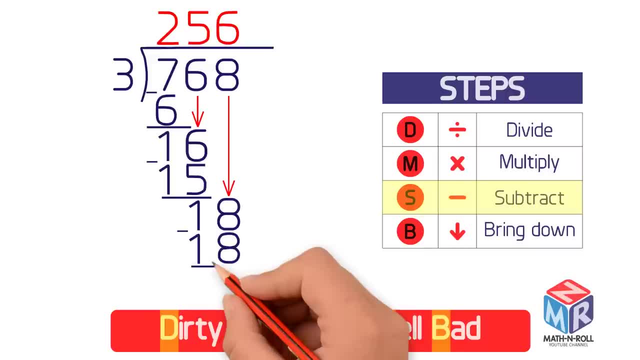 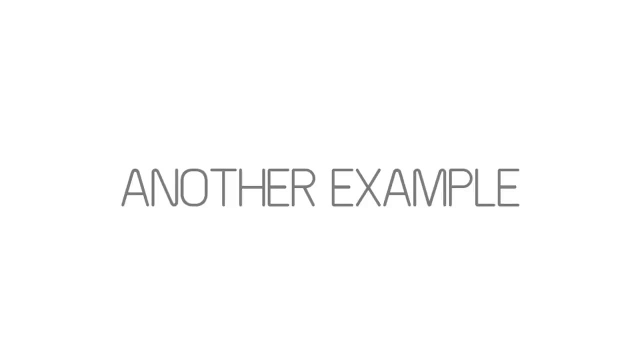 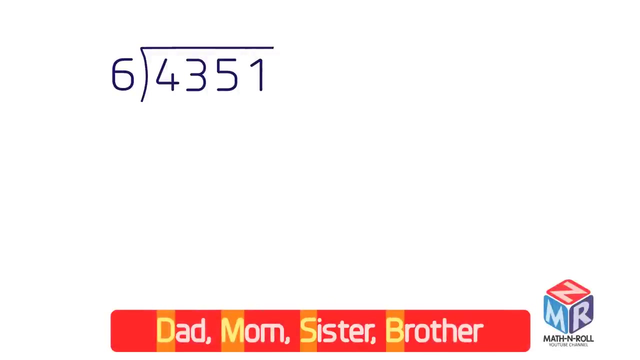 Now subtract 18 from 18 to get 0.. Because you have no more numbers to bring down, you are finished And the answer is 256.. Let's try another time. Let's try another example: Divide 4,351 by 6.. 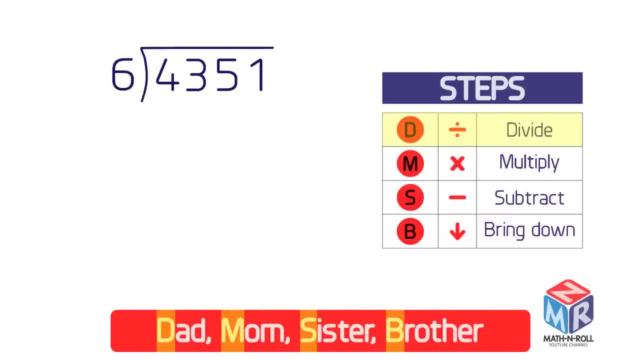 To begin ask how many times 6 goes into 4.. None, That's because the first digit taken by itself is less than the divisor. 4 is less than 6.. Write 0, or just leave a space above the 4.. 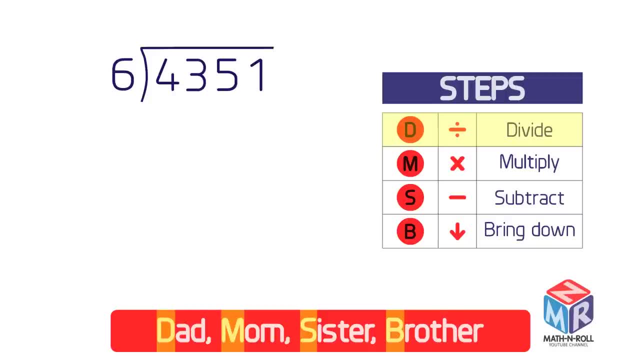 Let's group the 4 and the 3 together. Now ask how many times 6 goes into 43. That is, what's 43 divided by 6?? The answer is 7, with a little left over. So write 7 directly above the 3.. 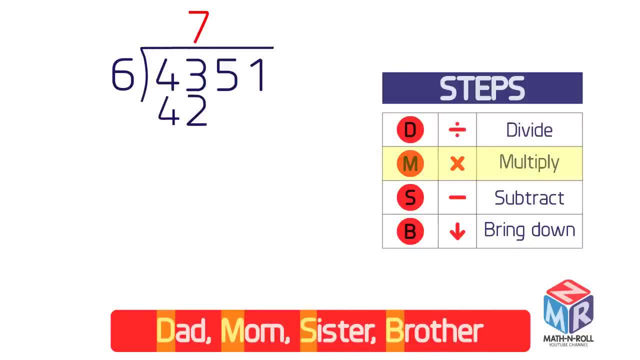 Now multiply 6 by 7 to get 42.. Place the product directly below the 43. And draw a line beneath it. Subtract 42 from 43 to get 1.. After you subtract, the result should be less than the divisor. 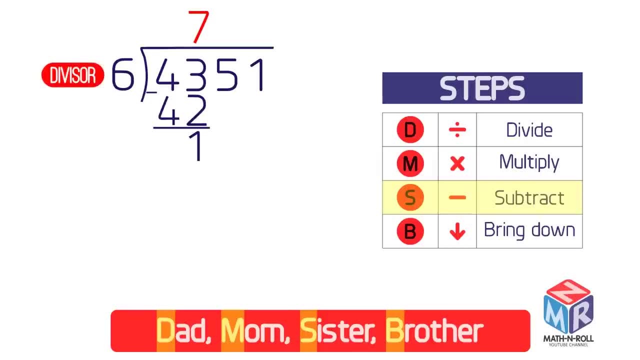 1 is less than 6, so it's okay. Then bring down the next number, 5, to make the new number 15.. Now ask how many times 6 goes into 15.. That is what's 15 divided by 6?. 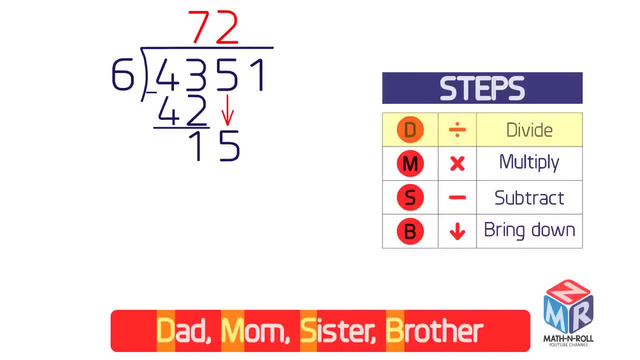 The answer is 2. Leave the remainder, So write the 2 above the 5, and then multiply 6 by 2 to get 12.. Write the product under 15.. Subtract 12 from 15 to get 3.. 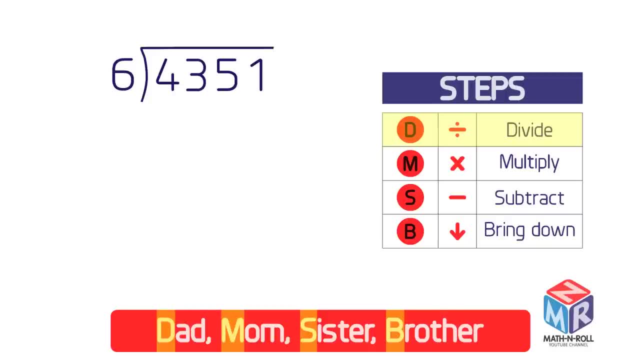 Now ask how many times 6 goes into 43. That is, what's 43 divided by 6?? The answer is 7, with a little left over. So write 7 directly above the 3.. Now multiply 6 by 7 to get 42. 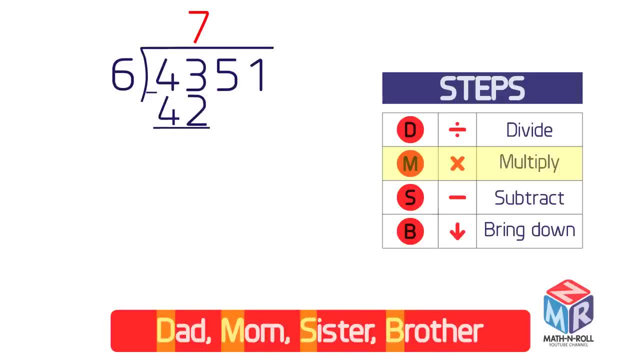 Place the product directly below the 43, and draw a line beneath it. Subtract 4,351 by 6, and place this below the 43. That's because the first digit, taken by itself, is less than the divisor. Subtract 42 from 43 to get 1.. 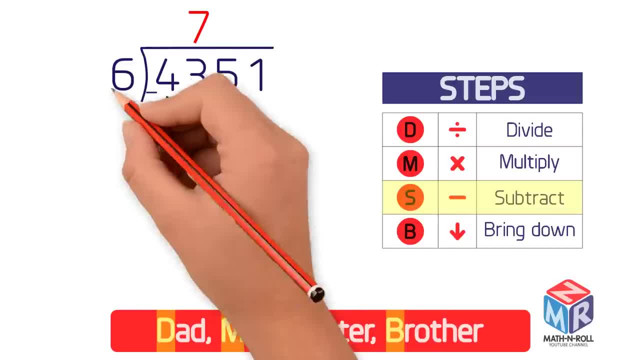 After you subtract, the result should be less than the divisor. 1 is less than 6, so it's okay. Then bring down the next number, 5, to make the new number 15.. Now ask how many times 6 goes into 15.. 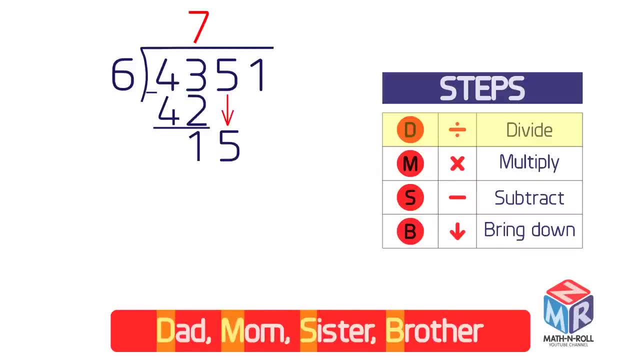 That is, what's 15 divided by 6?? The answer is 2, with a remainder. So write the 2 above the 5. And then multiply 6 by 2 to get 12.. Write the product under 15.. 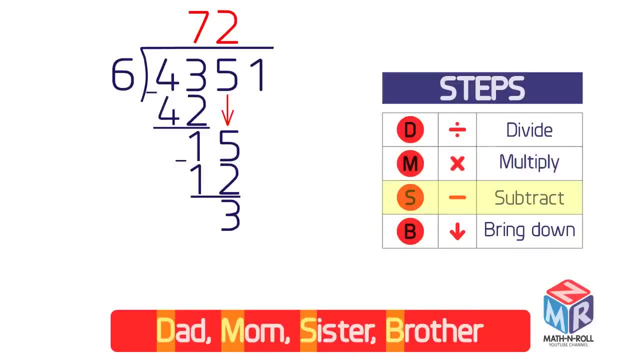 Subtract 12 from 15 to get 3.. After you subtract, the result should be less than the divisor. 3 is less than 6, so it's okay. Then bring down the next number 1, to make the new number 31.. 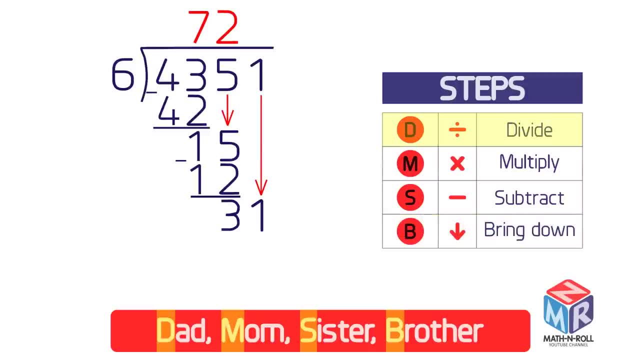 Another cycle is complete, So begin the next cycle by asking how many times 6 goes into 13.. That is, what's 31 divided by 6?? The answer is 5, with a remainder, So write the 5 above the 1.. 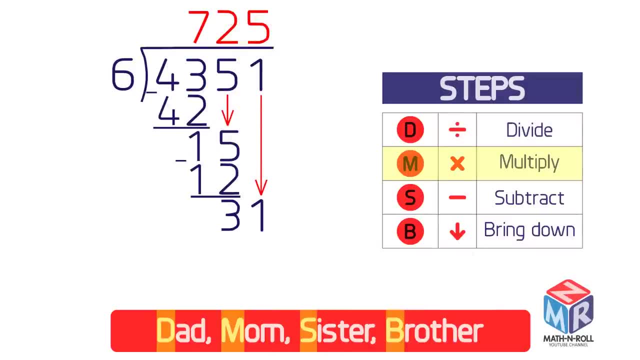 And then multiply 6 by 5 to get 30. Write the product under 31.. Now subtract 30 from 31 to get 1.. You have no more numbers to bring down. One is the remainder. You are finished. The answer is 725, with the remainder of 1.. 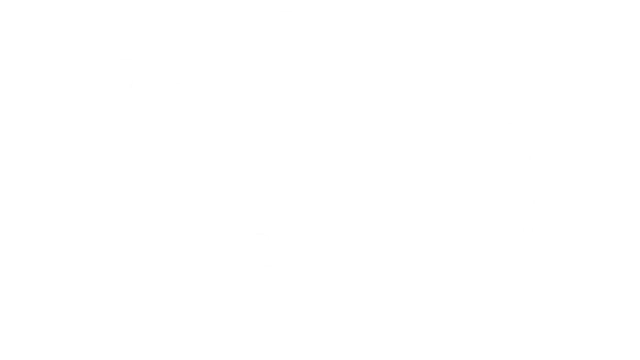 If you liked this video, please leave a like. For more videos like this, please subscribe.